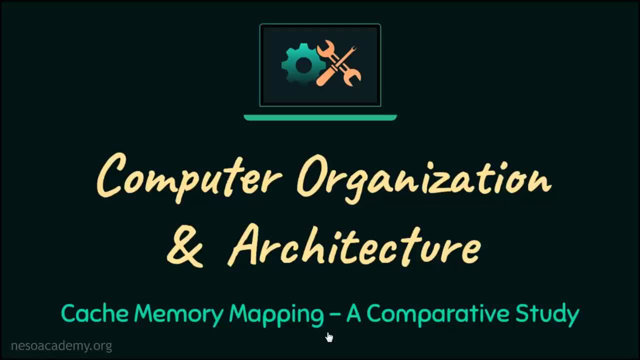 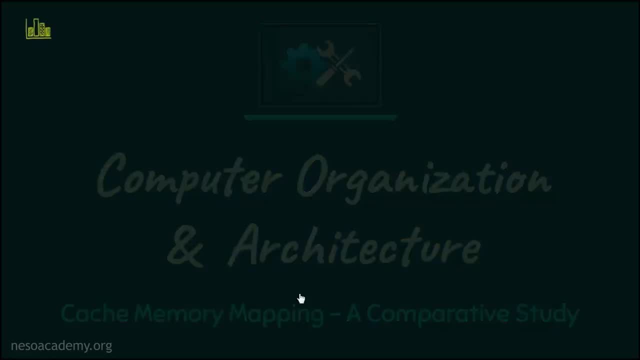 the distinctive natures of different kind of cache and memory mapping technique with the help of a constructive illustration. So without any further ado, let's get to learning. Suppose we are provided with some data. there is a main memory of size 8 gigabytes is given. 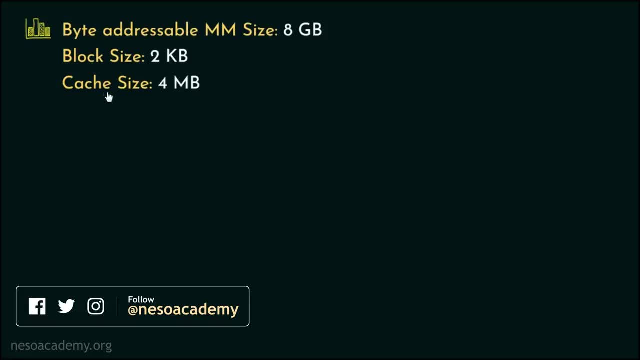 the block size is specified as 2 kilobytes and the cache is given of the size 4 megabytes. Now, since the memory is byte addressable, we know we need to change all the units into their respective bytes. Therefore, the main memory size is going to be 2 to the power. 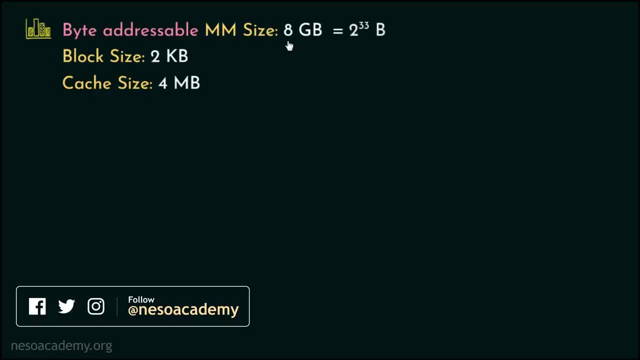 33 in terms of bytes, It is two cube and gigabytes is 2 to the power, 30. Therefore, for physical address, we will be needing 33 bet. Now coming to the block size, that is 2 kilobytes, which is, in terms of byte, is 2 to the power. 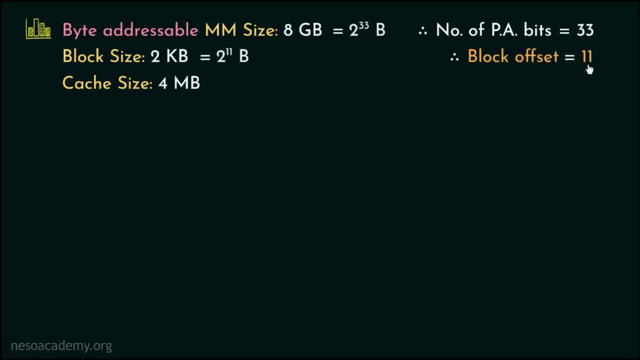 11.. Therefore, for block offset we will be needing 11 bits. know the cache size is given as four megabytes, which, in terms of bytes, is 2 to the power 22, because God is too square- and megabytes is 2 to the power 20.. 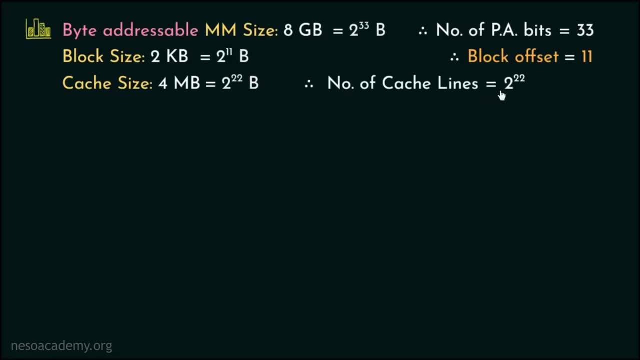 Now we can find out the number of caching lines. dividing the caching size 2 to the power 22 by the block or the line size, that is, 2 to the power 11, which will give us 2 to the power 11, because 22 minus 11 is 11.. therefore, there are 2 to the power 11 lines. 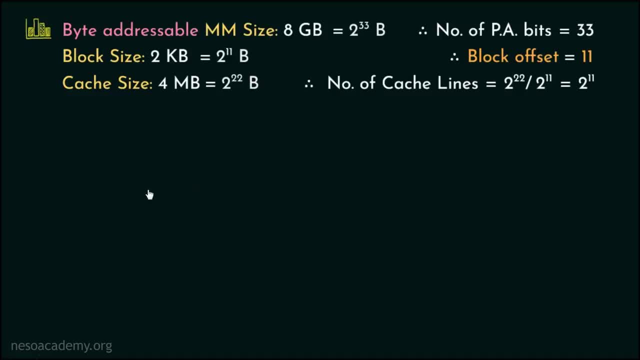 inside the cache. now let's observe what will be the physical address split in terms of direct associative and set associative mapping respectively. now we know: for physical address, we will be needing 33 bits and the block offset is of 11 bits, which will remain the same for all. 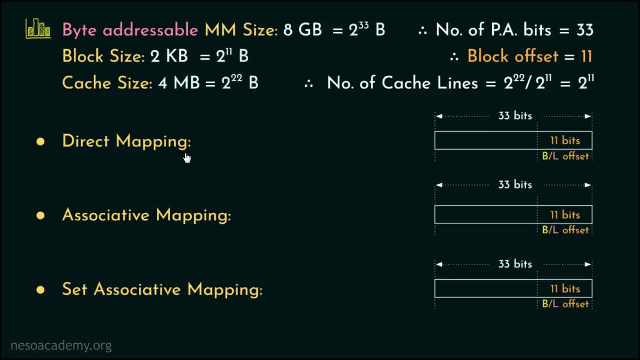 the different memory mapping techniques. now coming to the direct mapping, we already know there are 2 to the power 11 number of lines inside the cache. therefore, 11 bits are going to be used for the line number portion. now, since we are dealing with direct mapping, we know the number. 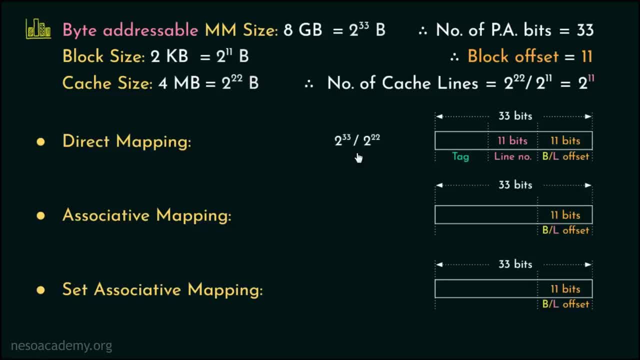 of tag bits can be found out from the ratio between the main memory and the cache memory size, which will give us 2 to the power 11, specifying that 2 to the power 11 main memory blocks will be mapped onto the each of the cache lines. therefore, the number of the cache lines 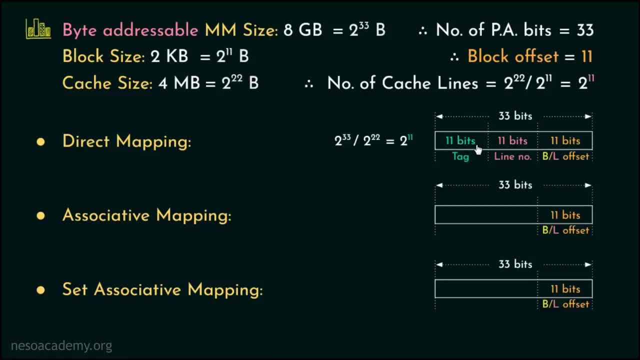 and the number of tag bits is nothing but 11 bits. so, from 33 bits physical address, 11 most significant bits will be used for the tag, 11 bits will be used for the line number and the 11 least significant bits will be used for block or line offset. now coming to associative mapping, we know 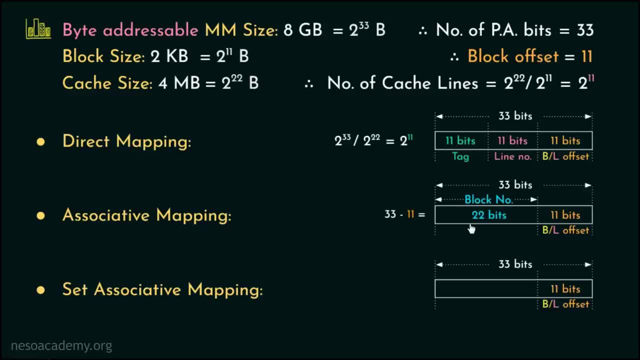 for the entire block number we will be needing 33 minus 11, that is, 22 bits. and since there are no restrictions about placing the main memory blocks into the cache lines, we also know that top number bits will be used for the tags. now let's talk about the physical address plate in. 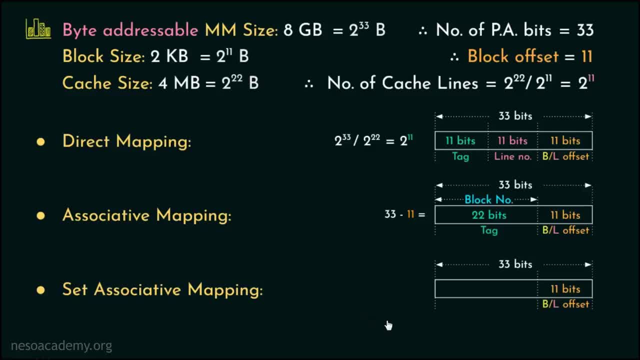 terms of set associative mapping. now, we also know that we can't really find out the ps plate if we don't really specify the way in set associative mapping. therefore, arbitrarily, let's assume it's a four-way set associative mapping. now, since it's a four-way, we know every set is going to. 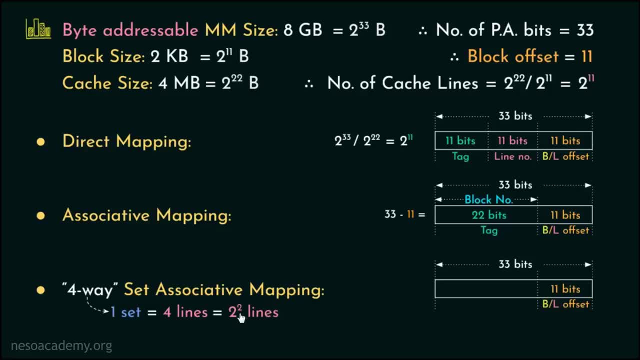 have four lines in them, that is, two to the power, two or two square lines inside every set. the number of sets can be found out dividing the cache lines, that is, 2 to the power 11, by the set size, which is 2 square, which will give us 2 to the power, 9 bits. therefore, 9 bits are going to. 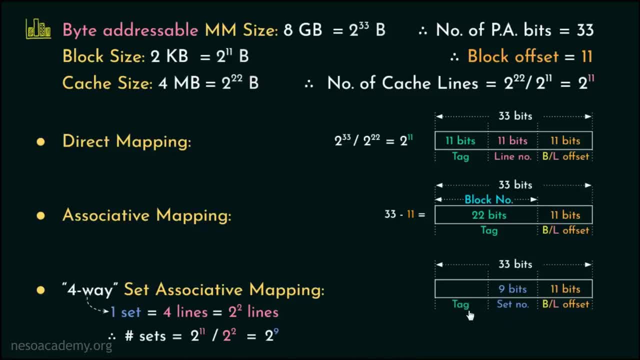 be used for the set number. and finally, for tag bits we will be needing 33 minus 9 plus 11, that is 20, that is 13 bits. so these are the different physical address plate for direct associative and four-way set associative mapping. now let's try to find out the key. 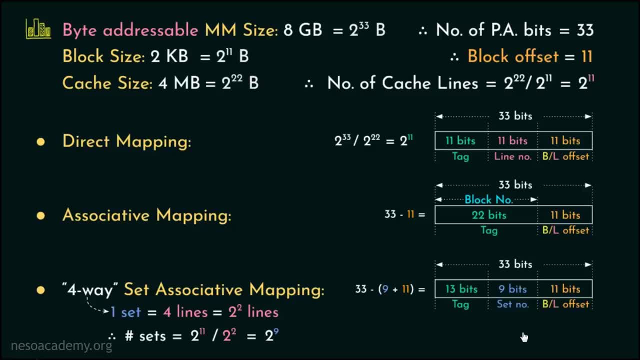 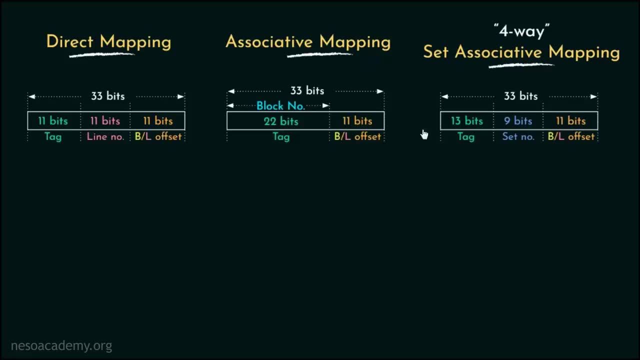 differences with the help of these physical address plates, shall we so? this is the physical address plate for direct mapping, this one is for associative mapping and this one we acquired for four-way set associative mapping from the same main memory and cache organization. now we will have a prominent understanding of this comparative 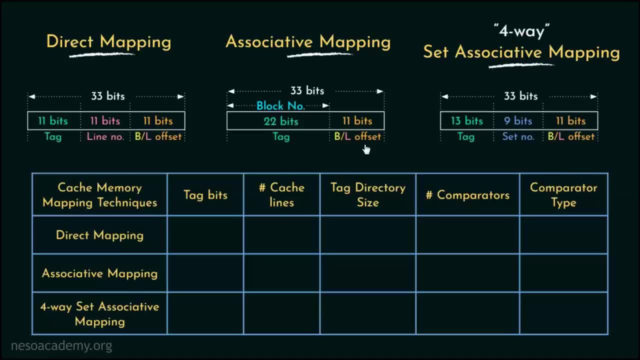 study with the help of this chart. as you can see, the parameters are kept column wise and the rows are there for different mapping techniques. now coming to tag bits, which is used for the identification of the main memory blocks inside the cache lines. in direct mapping, we are using 11 bits. in associative mapping, we 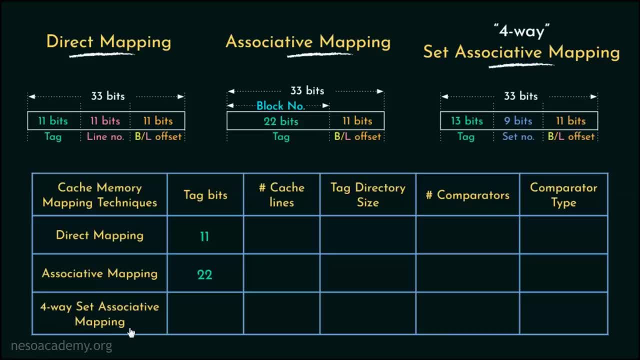 are using 22 bits, and for four-way set associative mapping, 13-bit stacks are used. now. the number of the cache lines is a sole property of the cache. that, too, depends on the size of the line or the block, and it has got nothing to do with the cache. 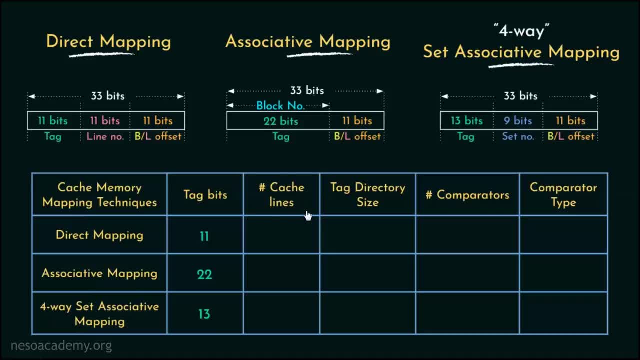 techniques. therefore, the number of cache lines will remain the same for all the different cache memory mapping techniques, which we calculated to be 2 to the power 11.. now, coming to the tag directory size, we know the number of tag directory entries will be as same as the number of cache lines are. 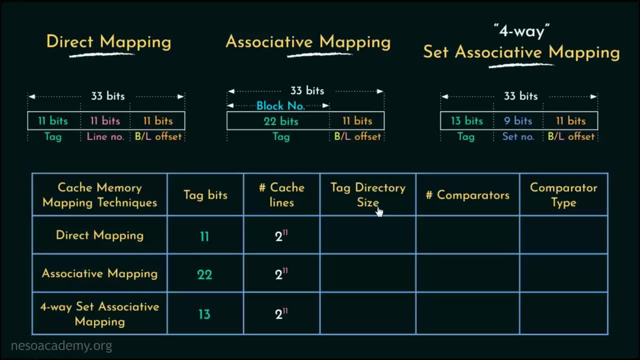 in there. however, the tag directory size altogether will vary because of the different number of tag bits in different mapping techniques. therefore, for direct mapping, the size of the tag directory is going to be 2 to the power 11 multiplied by 11 tag bits. now coming to associative mapping, the 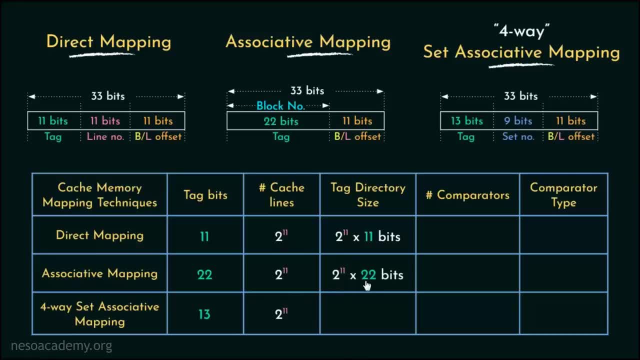 tag directory size will be 2 to the power 11 multiplied by 22 tag bits. similarly, in case of four-way set associative mapping, the size of the tag directory will be 2 to the power 11 multiplied by 13 tag bits. now, as you can see, the number of tag directory entries in every case is going to. 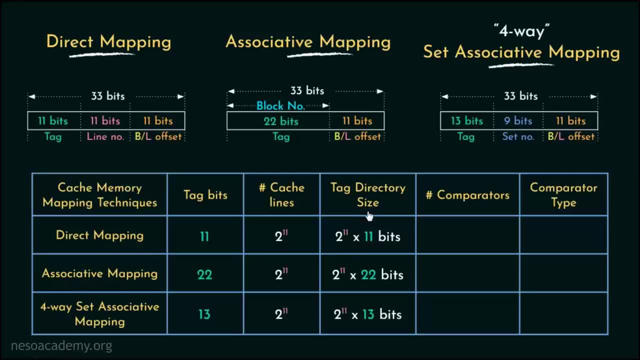 be the same. however, the tag directory size will differ because of the different tag bit size. now let's talk about how many number of comparators we are going to need for different mapping techniques. coming to direct mapping, we already know it's a very strict mapping policy and for block identification, we are going 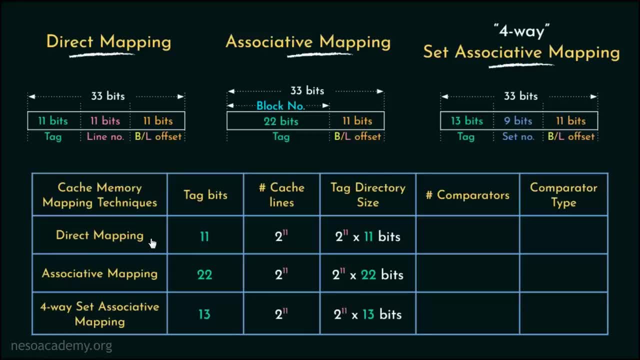 to compare only a single cache line at a time. therefore, for direct mapping, the number of comparators we will be needing is only one, whereas in case of associative mapping we already have all the cache dependency to do all the static Independently. that means we don't have any. 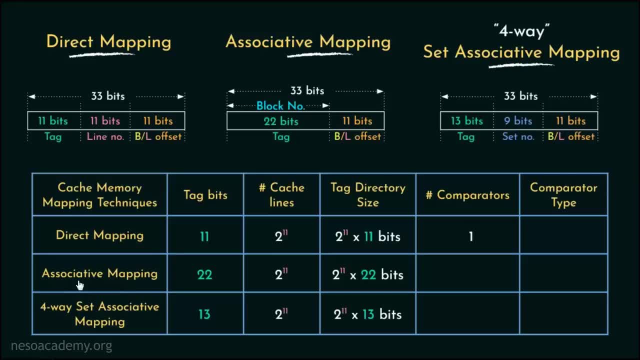 restrictions on placing any of the main memory blocks into any of the cache lines. therefore, for associative mapping we will be needing 2 to the power 11 number of comparators, because we need the comparators to be associated with all the cache lines, and hence 2 to the power 11 number. 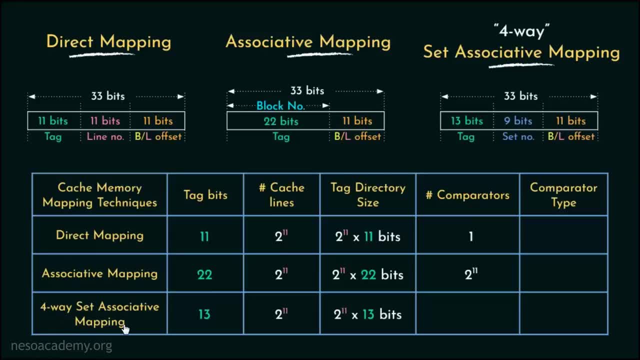 of comparators. now coming to four-way set associative mapping, we know, due to the four-way, every set inside the cache is going to have four lines in them them. That means we will be comparing only four lines belonging to the same set during block identification. Therefore, the number of comparators we will be needing for four-way set associative 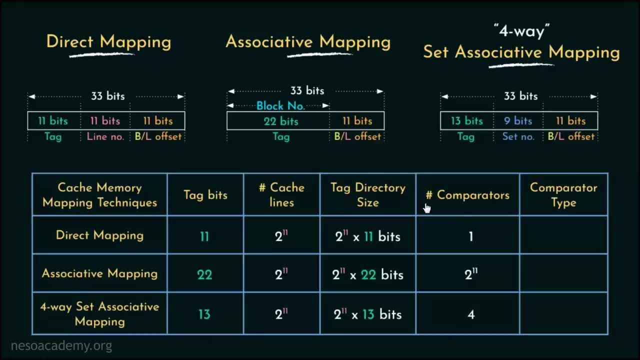 mapping is going to be four. So, to summarize, the number of comparators needed for direct mapping will always be one. Coming to associative mapping, it will be as same as the number of cache lines are in there. and coming to k-way set associative mapping, it will be depending on the value of k. 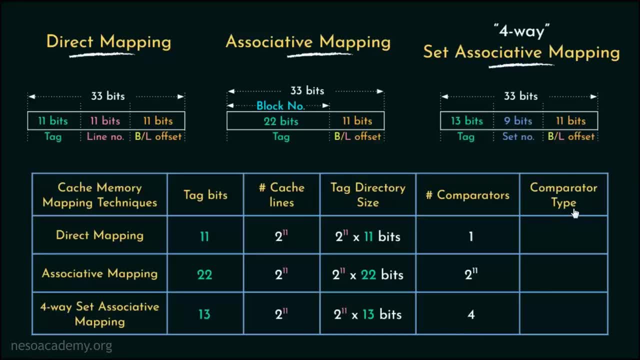 which is, in this case, is four. Now, coming to the type of the comparators, it totally depends upon the tag size, because comparing the tags associated to the cache lines with the tag field of the physical address, we can actually specify either the block's presence or absence inside the cache. 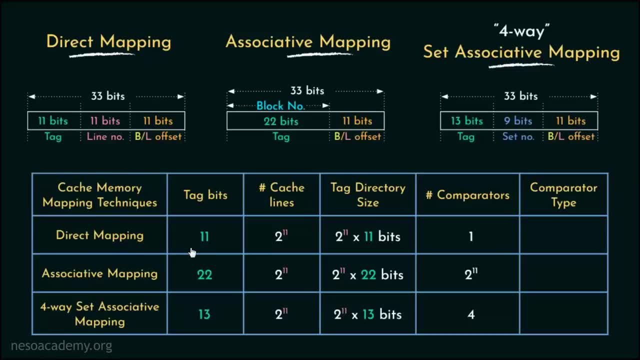 So, in this specific scenario, for direct mapping, we calculated the tag bits to be 11 bits. Therefore, we will be needing one 11-bit comparator, whereas in case of associative mapping, since the tag bits are of 22 bits, we will be needing two to the power. 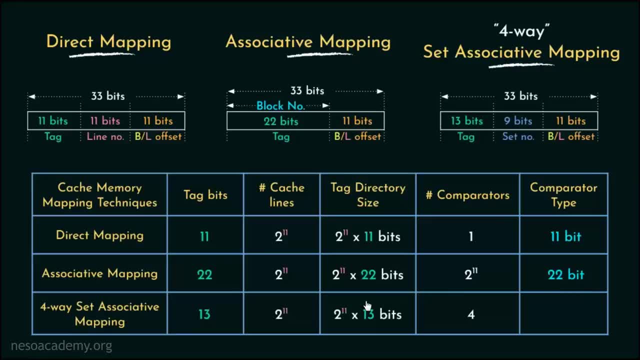 11 22-bit comparators. Similarly, for four-way set associative mapping, the tag size is of 13 bits. Therefore, we will be needing four 13-bit comparators. So these are the differences of different cache memory mapping techniques. Nonetheless, do always remember that the number 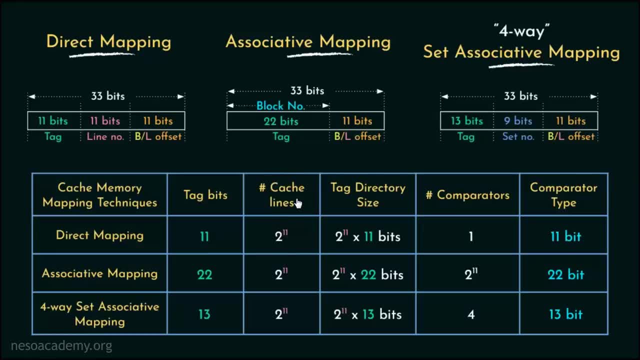 of lines inside the cache depends solely upon the cache line size. So in this case we will be needing the number of lines inside the cache's overall size and the block or the line size. So it has got nothing to do with different memory mapping techniques and that's why it remained the same. 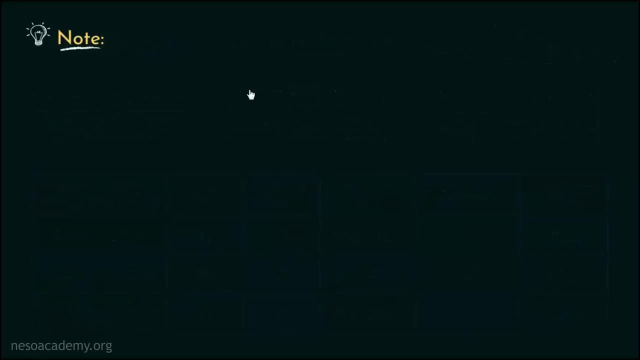 for all of them. Now, on a special note, we have already talked about set associative mapping as a combination of both direct and associative mappings. positive features In continuation of that discussion for a k-way set associative mapping if the value of k is one that means. 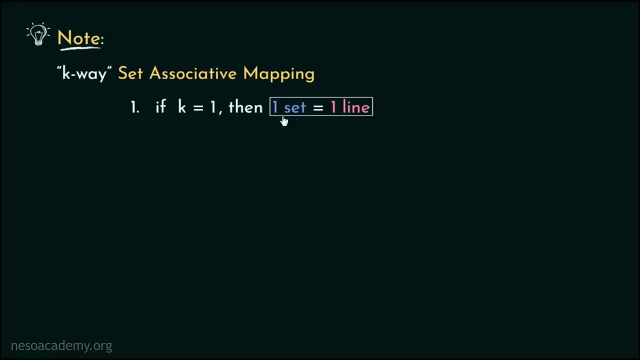 going to have a single line. that means every line is a set. In that case it is as same as direct mapping, because in direct mapping every main memory block is mapped onto a specific cache line. On the other hand, if the value of k is n, where n being the number of lines inside the cache,